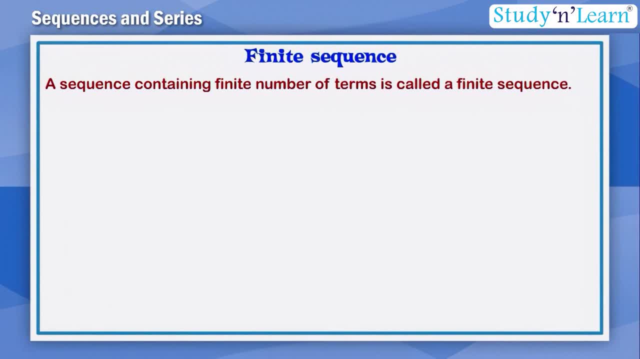 A sequence containing finite elements. A sequence containing finite elements, finite number of terms, is called a finite sequence. Now let us see what is an infinite sequence. The sequence is called infinite if it is not a finite sequence. That means the number of terms is not countable. 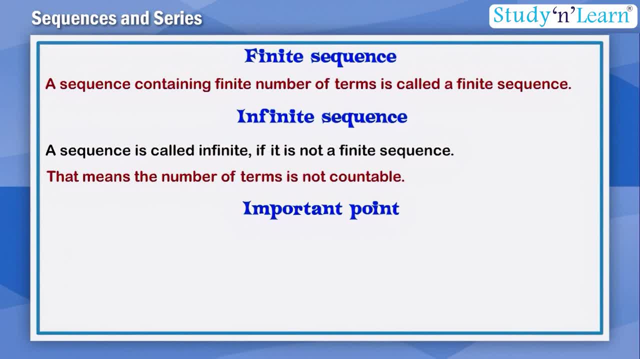 A very important thing about sequences is that in every sequence, we should not expect that its terms will necessarily be given by a specific formula. That is not. every sequence follows a definite pattern. However, we expect a theoretical scheme or a rule for generating the terms a1,, a2, a3 till an, and so on in succession. 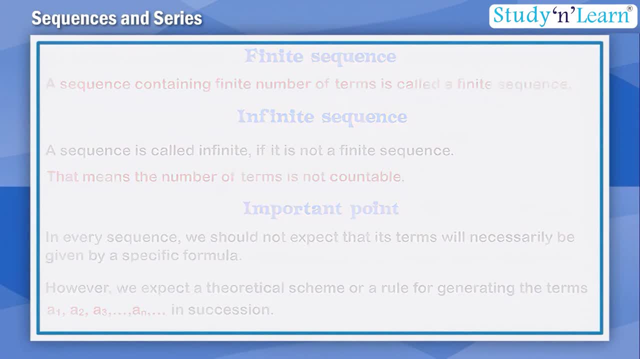 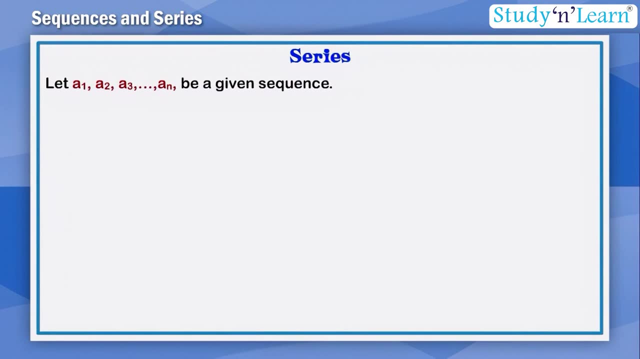 Now let us learn about series. Let a1, a2, a3 up to an be a given sequence, Then the expression a1 plus a2, plus a3, plus so on, till plus an plus so on, is called the series associated with the given sequence. 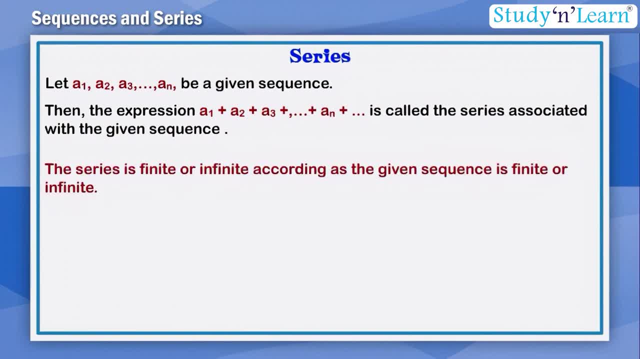 Subtitles by the Amaraorg community. The series is finite or infinite. according as the given sequence is finite or infinite, Series are often represented in compact form called sigma notation, using the Greek letter sigma as means of indicating the summation involved. Thus the series a1 plus a2 plus a3 plus so on till. 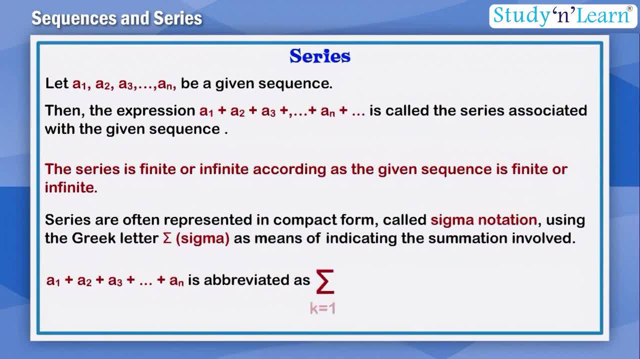 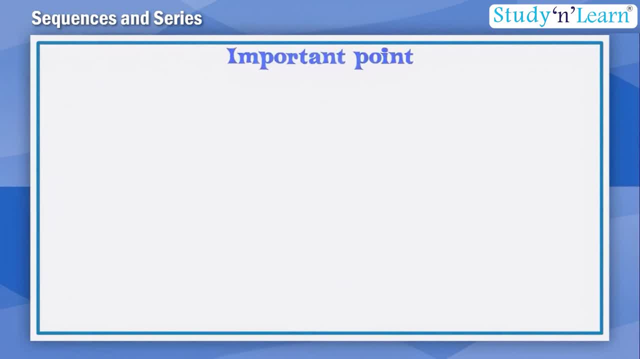 The series a1 plus a3 plus a3 plus, so on. till plus an is abbreviated as: summation k is equal to 1 till nak, An important point. When the series is used, it refers to the indicated sum, not to the sum itself. 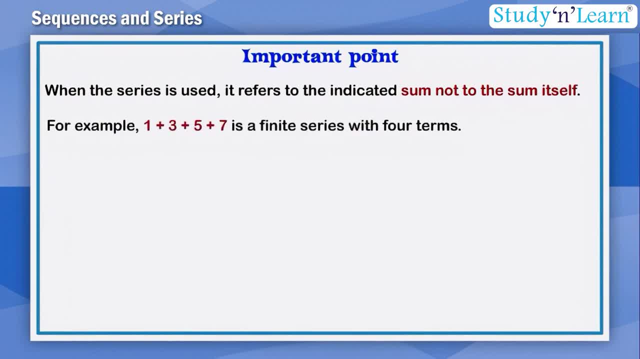 For example, 1 plus 3 plus 5 plus 7 is a finite series with 4. terms: However, when we use the phrase sum of a series, we will mean the number that results from adding the terms. the sum of the series is 16..